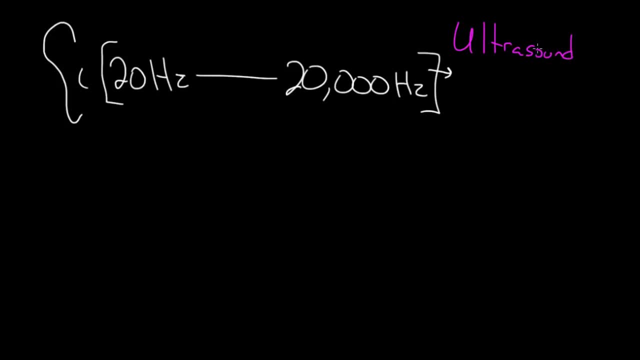 And this does more than just annoy animals. This has a practical purpose. If you wanted to image, do some medical imaging or figure out what's going on in the human body. So say, here's a portion of the human body and there's maybe a vital organ or some tissue here or some tissue over here, You're worried, something's going wrong. You've got to figure out what's going on inside. You can operate, but that obviously sucks. You want to try to avoid an operation if possible. You can do x-ray, but too much. 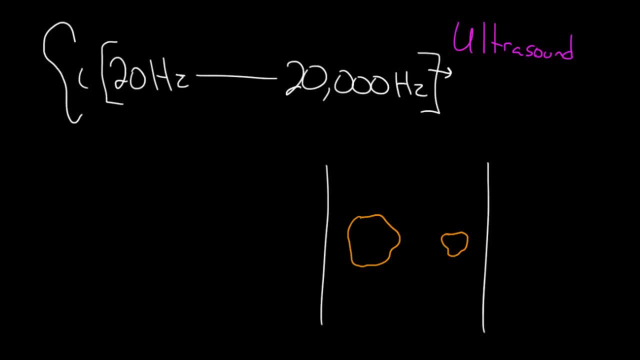 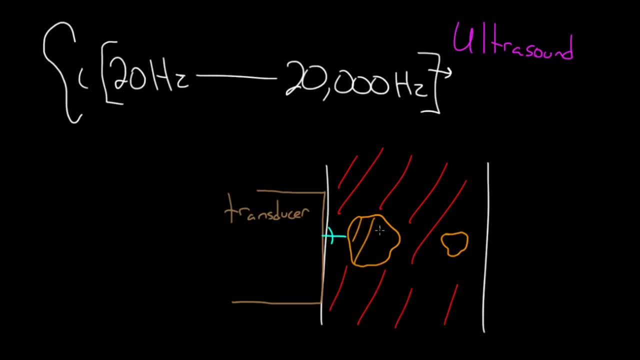 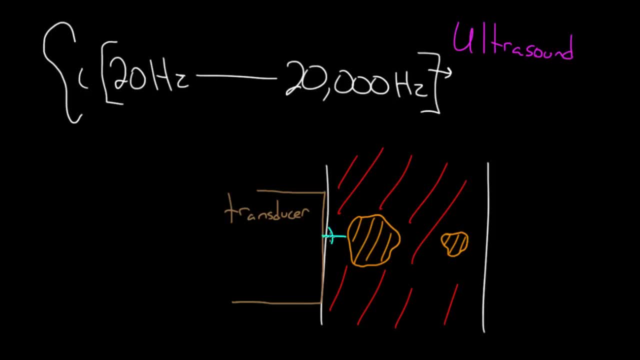 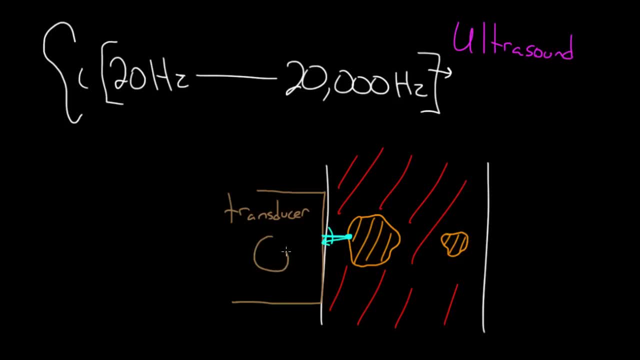 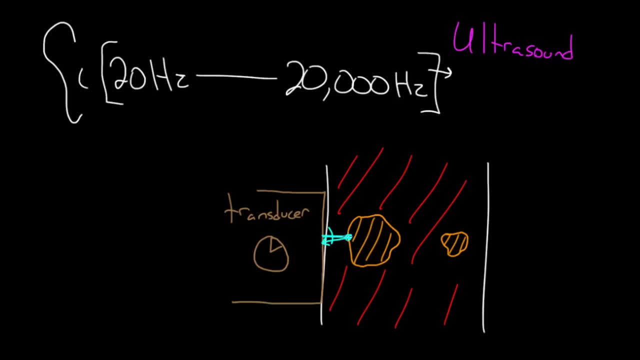 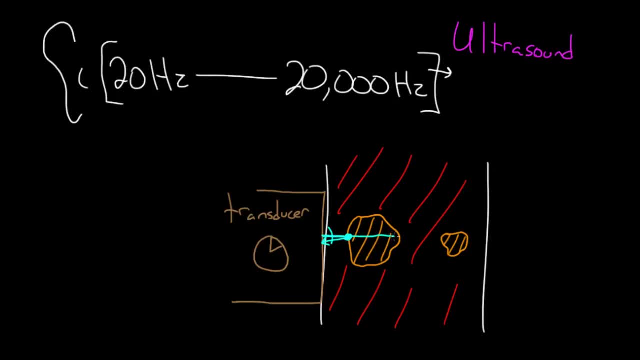 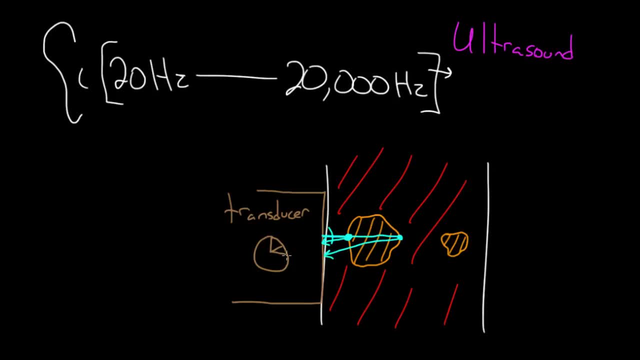 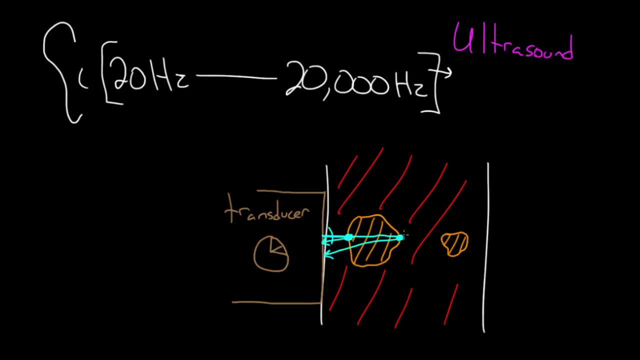 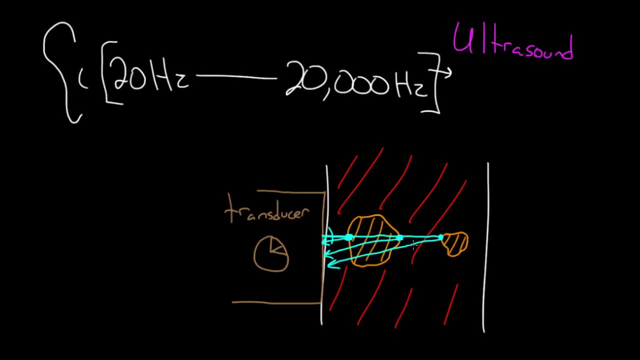 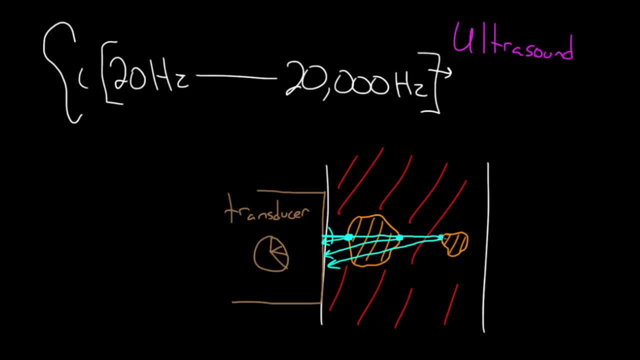 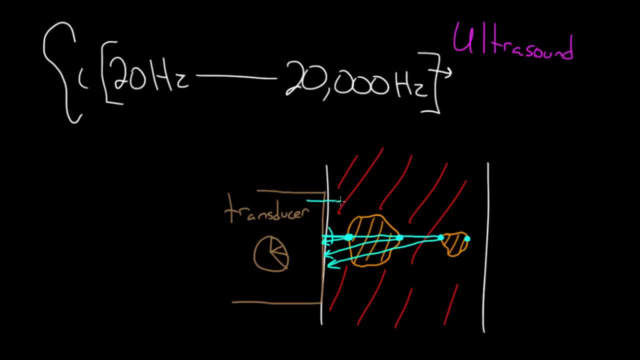 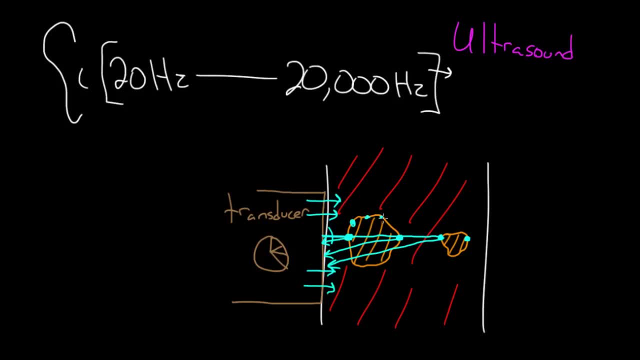 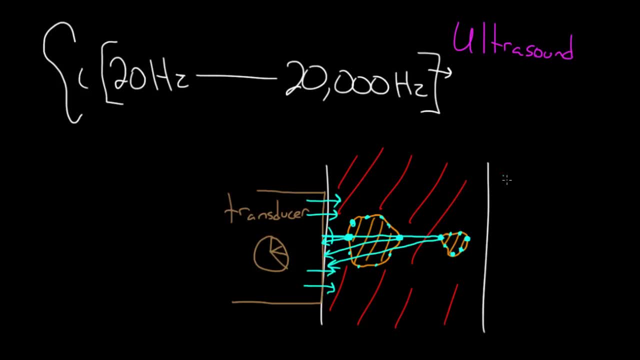 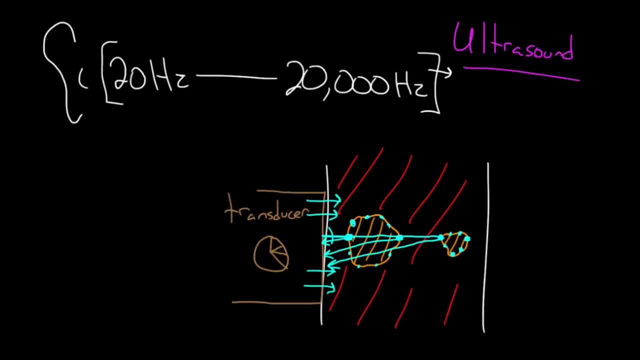 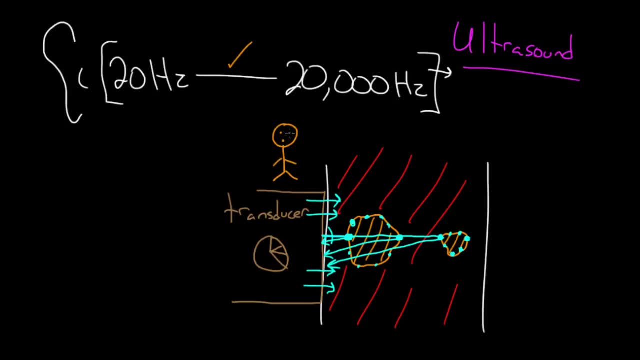 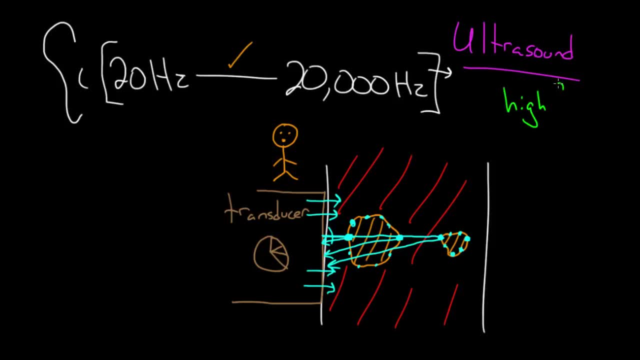 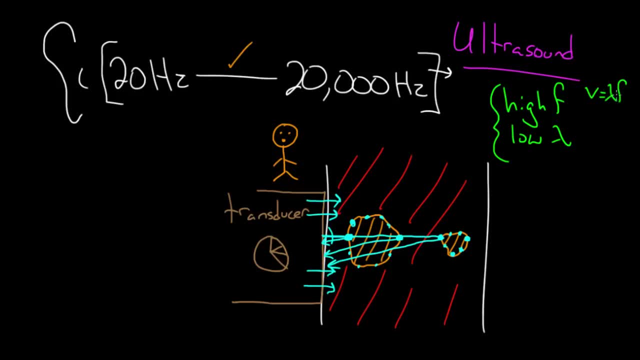 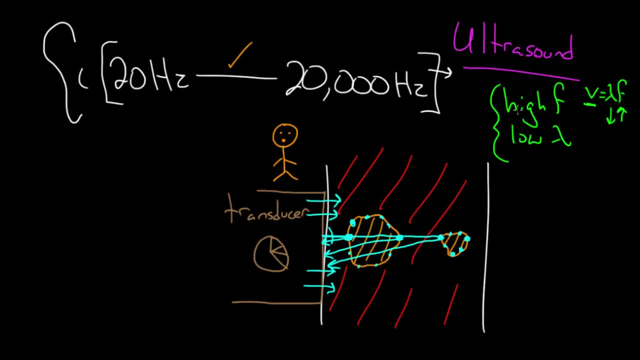